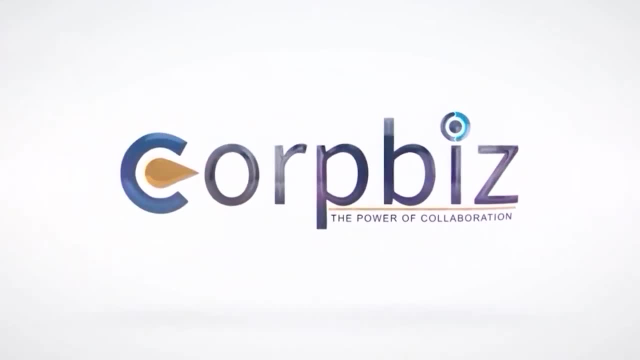 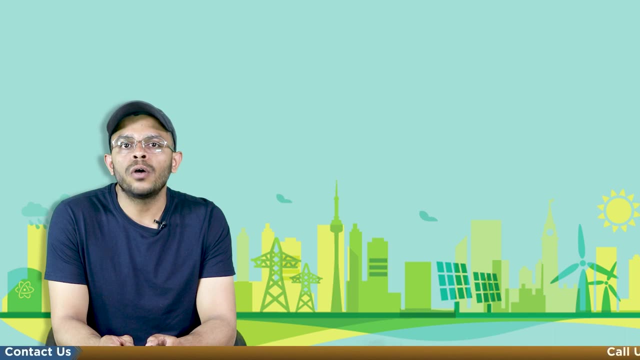 Hello and welcome to Copbiz. My name is Shaleen and today we will be learning about how an EIA report is made as per the guidelines issued by the Ministry of Environment and Forests. So, as you may know, the purpose of the EIA for any project is to obtain environmental clearance. 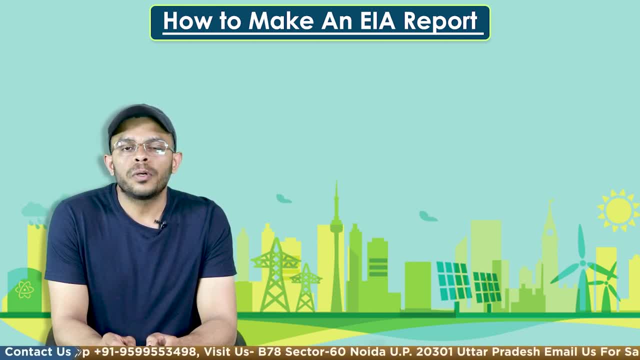 Road networks, water supply and management, energy production supply and management, communication services and many such infrastructural projects are all part of developmental projects. So at the time of selection of the site, the proponent must ensure that the land use status of the proposed area is consistent with the area's approved developmental plan. 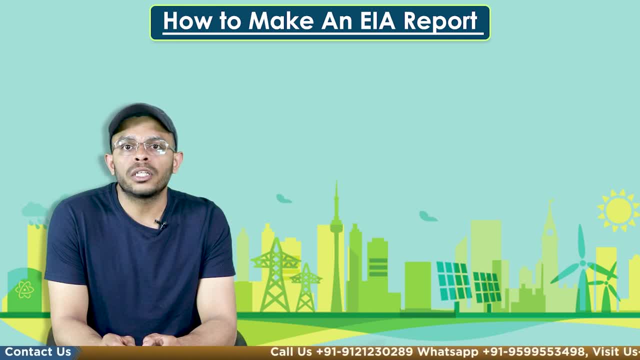 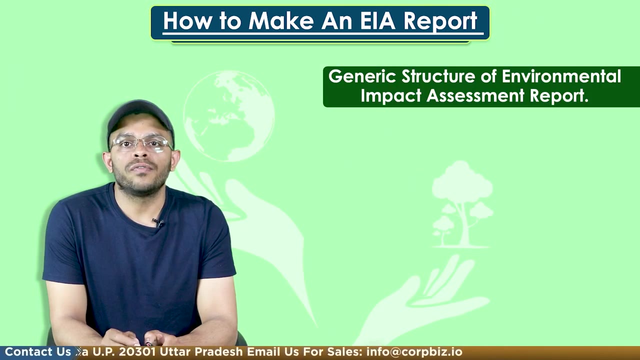 If no approved plan exists, the approval from the competent authorities should be obtained. Conducting an EIA is the next step. The projects that require an environmental impact assessment are designated as Category A and Category B, So let's understand the generic structure of the Environmental Impact Assessment Report. 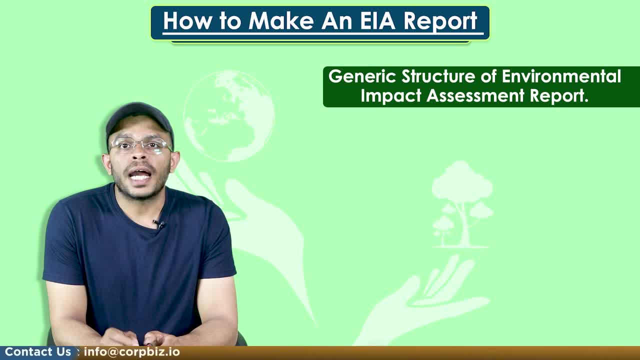 According to the Ministry of Environment and Forests, the EIA guidelines were issued in 2006 for developmental projects. Now, the generics format of the EIA document should include the following: Introduction: Projects Description. Environmental Description: Anticipated Environmental Impact Assessment. 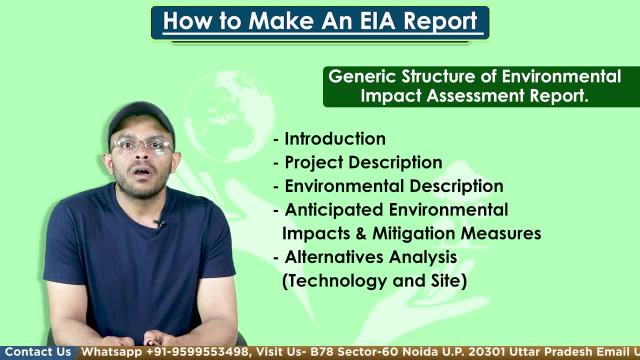 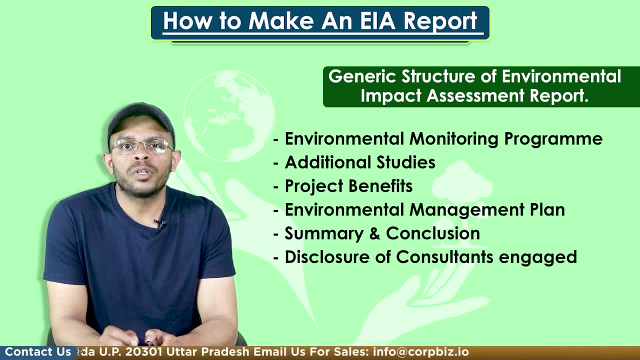 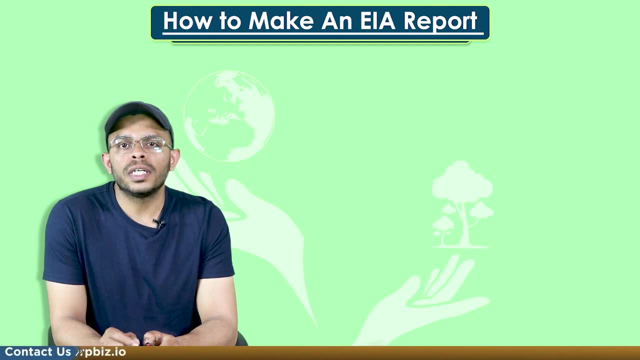 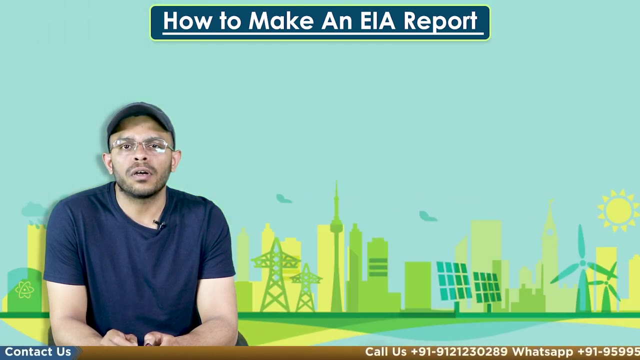 Introduction, Projects Description, Environmental Description, Anticipated Environmental Impact Assessment, Domination of product impacts & mitigation measures, Alternative analysis for technology and site Environmental monitoring program, Additional studies, Project's benefits, Environmental Management Plans, Summary & Conclusions. So when we talk about the composition of the above format, details like the project proponents, profile, contact information, brief description of the projects, etc. must be included. 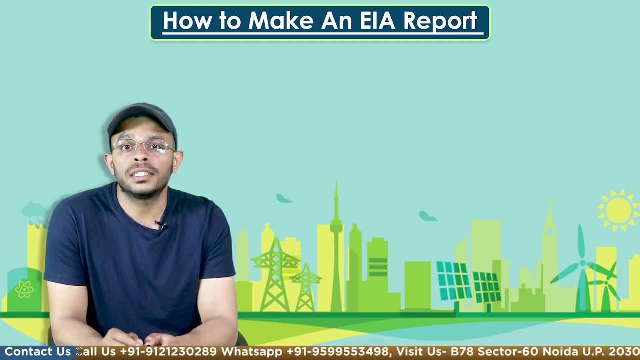 In this section, the details of a project, as its nature, size, location and its significance to the country and the area must be mentioned. An action plan must be properly described in terms of existing national and international environmental laws, If any restrictions or limitations are imposed by the district. 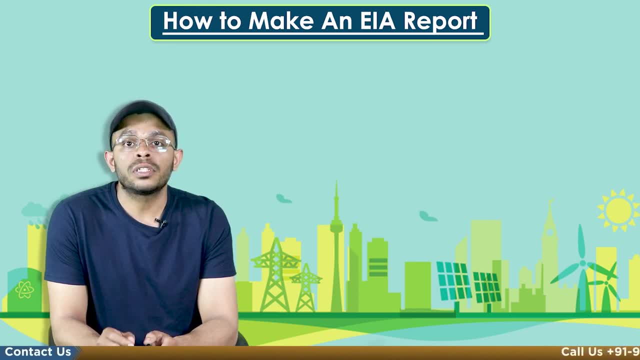 administration, state or the central government. they must also be included. Details of any litigation pending against the project or the project site in any court should be provided. In the event of project's expansion or modernization, the environmental compliance status for the current project should be provided. Let's see the documents that are required in case. 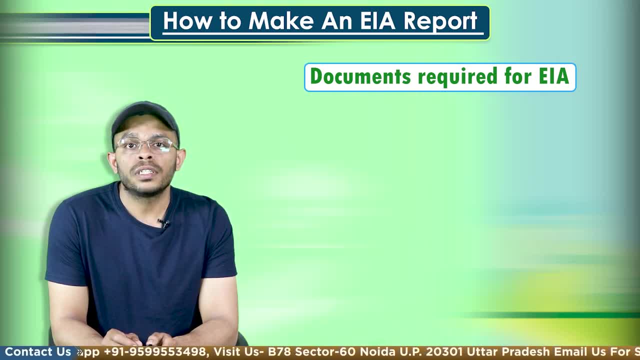 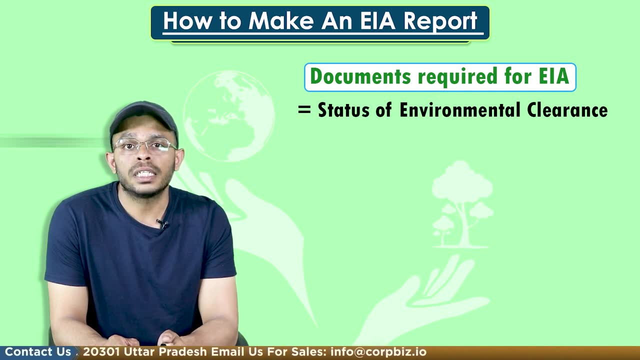 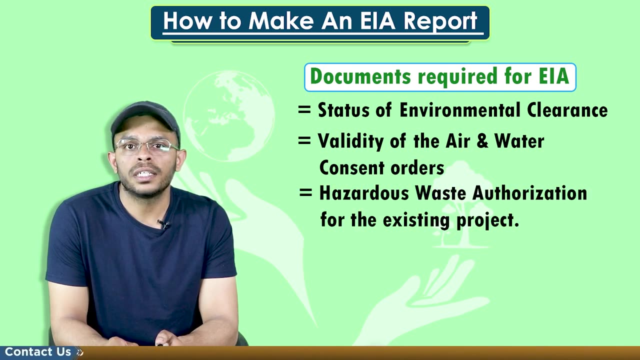 an EIA is needed for a development project. First is the status of environmental clearance and compliances with the terms and conditions for the existing project. Next is the validity of the air and water consent orders. Next is hazardous waste authorization for the existing project. Next comes the notices and 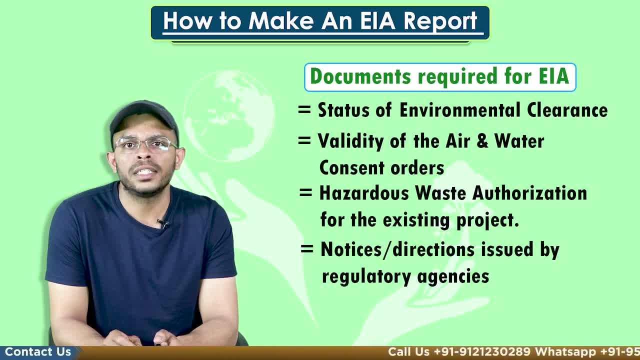 directions issued by the regulatory agencies under Section 33 of the Water Act and Section 31 of the Air Act during the last one year. Next is the identification of natural hazard-prone areas, such as earthquake-prone areas, cyclone-prone areas, flood-prone areas. 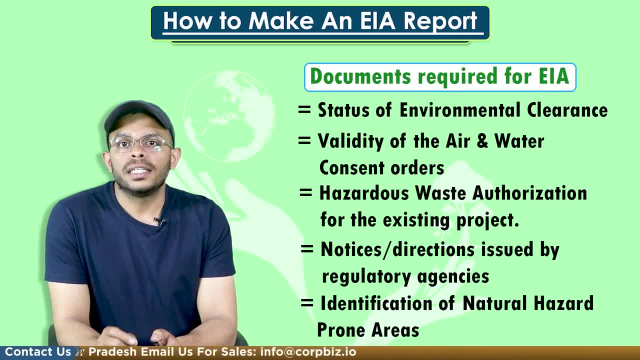 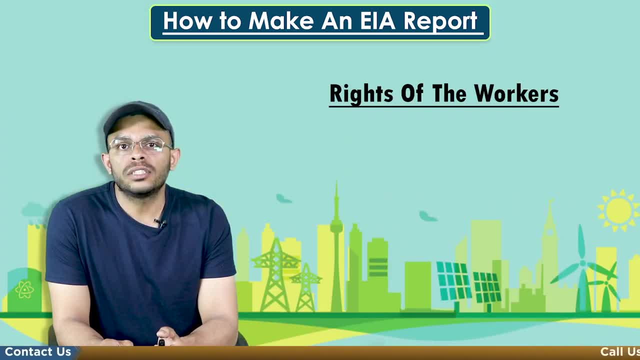 and landslide-prone areas. Let's understand the guidelines issued for development projects in different areas. First, let's talk about how the guidelines addresses the rights of the workers. To ensure the proper health and safety of construction workers, effective provisions for basic sanitation, drinking water and equipment or mechanical safety must be included as a part of 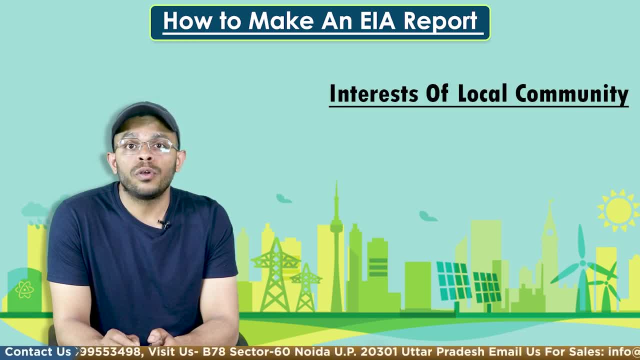 your EIA. Next is considering the interest of local community into account, So the guidelines for development projects insist on highlighting the advantages of the proposed project to the community, the region and the country. This section can also include beneficial details such as improvements from the project's infrastructure, as well as any auxiliary business that may emerge. 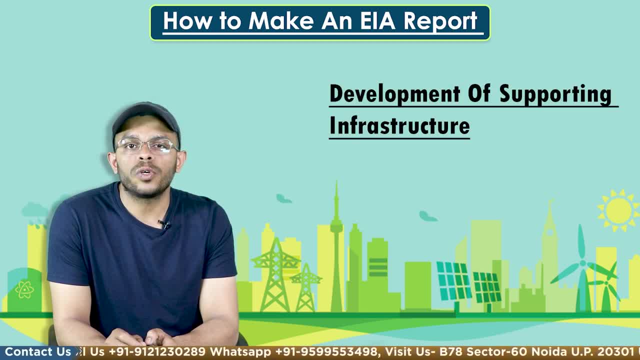 as a result of the project. Next is development of supporting infrastructure. As per the guidelines, the EIA must include improvements to social infrastructure such as roads, trains, townships, housing, water supply, electricity, drainage, education, institution hospitals, etc. Employment: 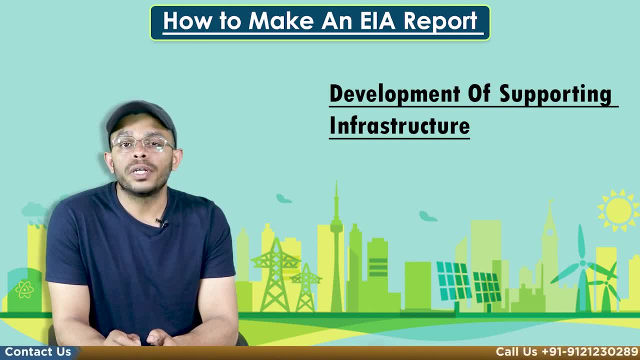 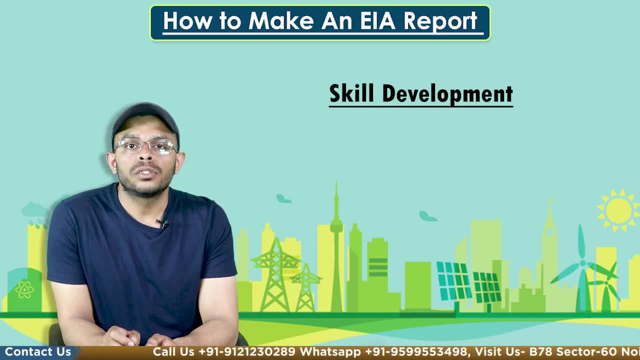 potential for skilled, semi-skilled and unskilled labour during the construction and the operation phase of the project must also be highlighted. Next is skill development, So special attention should be paid to the employment potential of the local population, as well as the requirement. 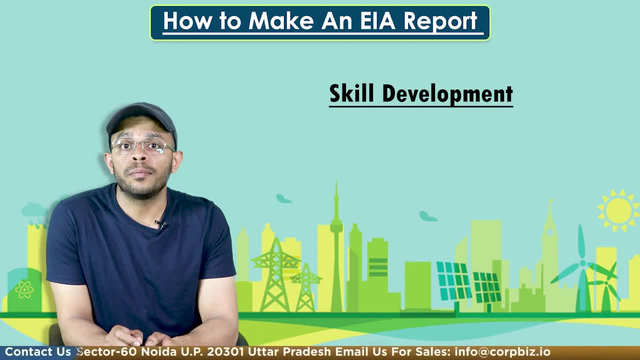 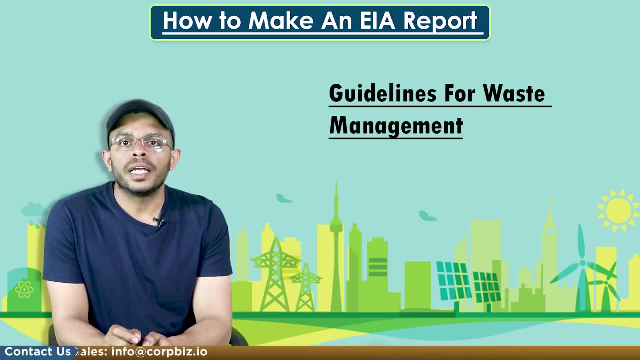 to impart relevant skills to them in order to train them to be eligible for such employments. The next in the guidelines is for the waste management. Proper waste management, including garbage collection, segregation, treatment, waste management, waste management, waste management, treatment and disposal should be included in the development project. Infrastructure maintenance.